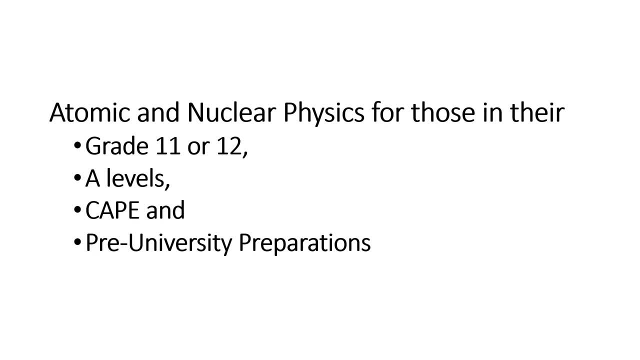 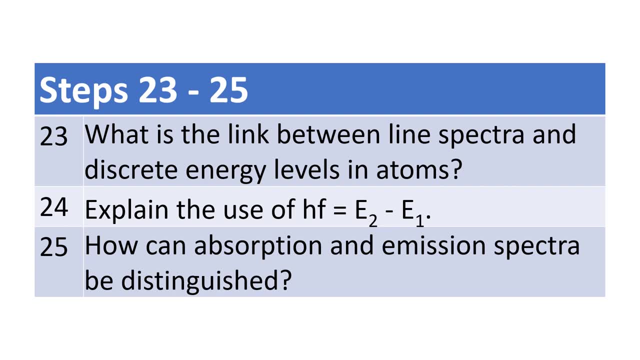 A-levels, CAPE and pre-university preparations, Steps 23 to 25.. 23. What is the link between line spectra and discrete energy levels in atoms? 24. Explain the use of HF equals E2 minus E1.. 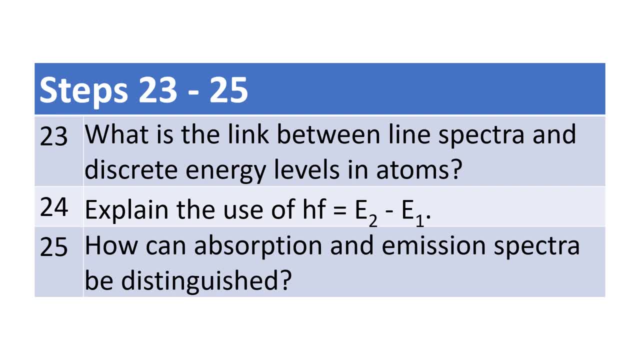 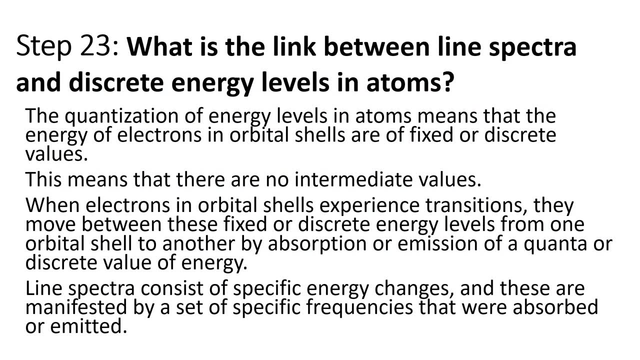 25. How can absorption and emission spectra be distinguished? Step 23. What is the link between line spectra and discrete energy levels in atoms? The quantization of energy levels in atoms means that the energy of electrons in orbital shells are of fixed or discrete values. This means that there are no intermediate values. 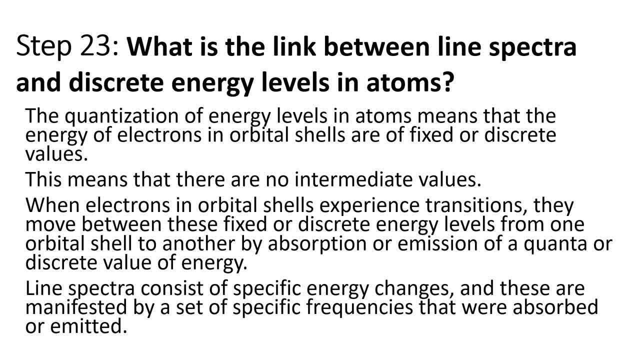 When electrons in orbital shells experience transitions, they move between these fixed or discrete energy levels from one orbital shell to another by absorption or emission of a quanta or discrete value of energy. Line spectra consist of specific energy changes, and these are manifested by a set of specific frequencies that were absorbed or 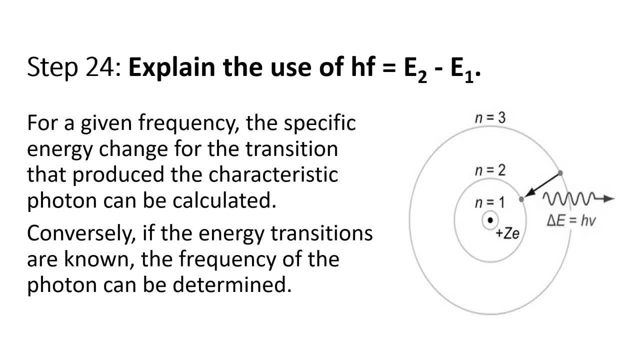 emitted. Step 24. Explain the use of HF. equals E2 minus E1.. For a given frequency, the specific energy change for the transition that produced E2 minus E1 is the transition that produced E2 minus E1.. Step 25.. How can absorption and emission spectra be distinguished? 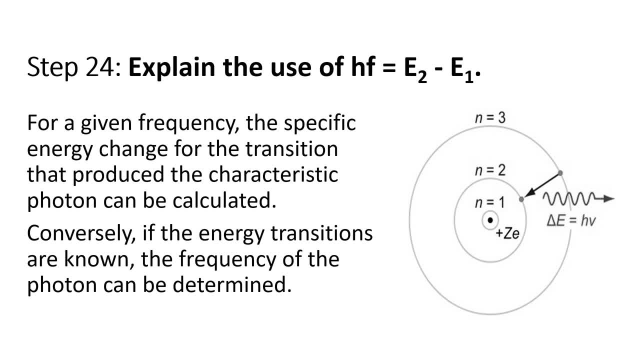 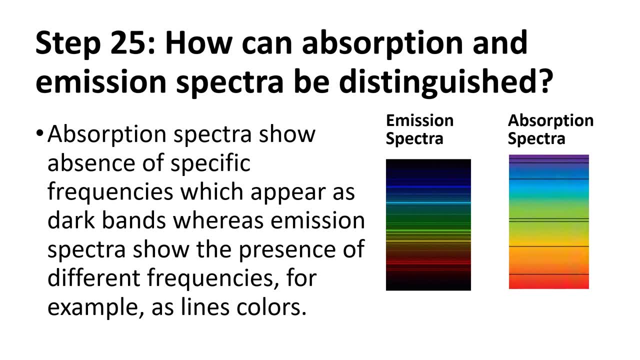 Step 26. Why? Conversely, if the energy transitions are known, the frequency of the photon can be determined. Step 25. How can absorption and emission spectra be distinguished? Absorption spectra show absence of specific frequencies, which appear as dark bands, whereas 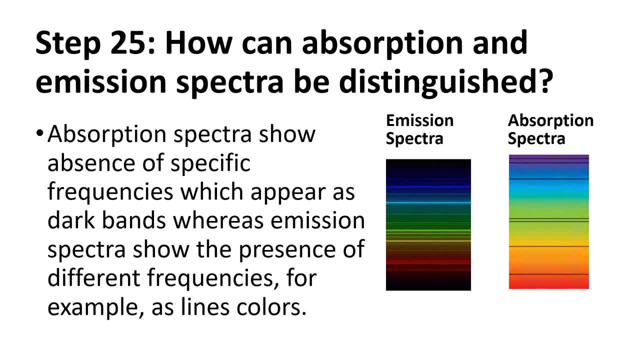 emission spectra show the presence of different frequencies, eg as lines of colors, Step 27. Why? Because emission spectra don't show the presence of O閃, aber ihrer events, in the soliciton of star energy and star news right after the birth andscheering of E2 minus E1 minus E2s. 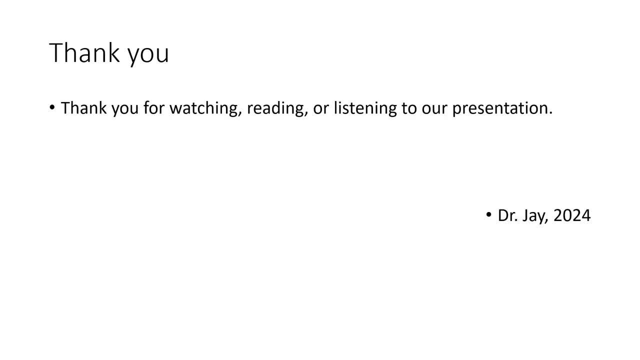 Step 28.. Why can emission spectra be distinguished? Step 29.. Why can high- América sparkняя so Falconja can value of 5 quietly, Thank you. Thank you for watching, reading or listening to our presentation, Dr J 2024..